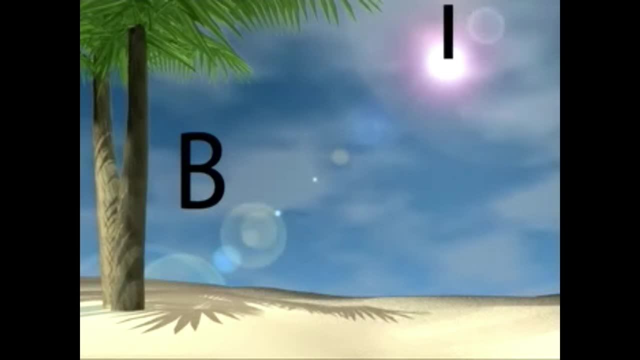 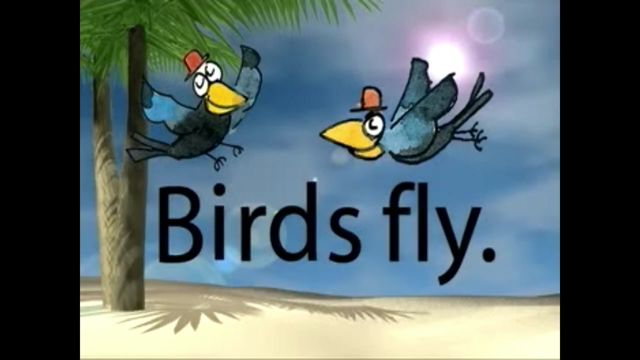 I am letter B. This is letter I. I am letter I, Letter R, letter D and letter S. When these five letters go together they make the word birds. If they bump into another word they may become a sentence. 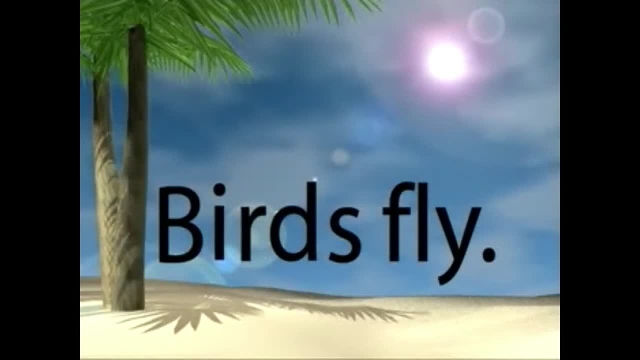 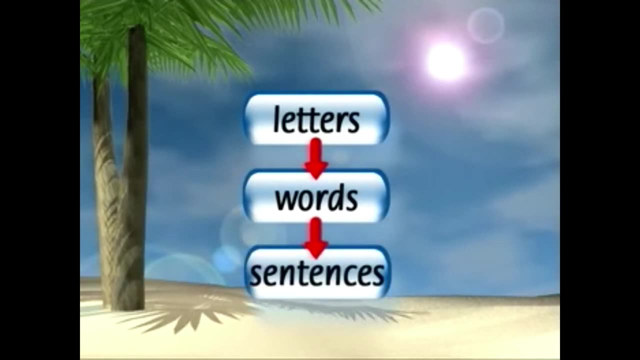 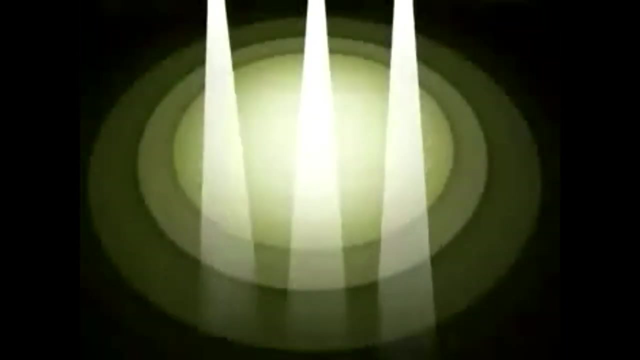 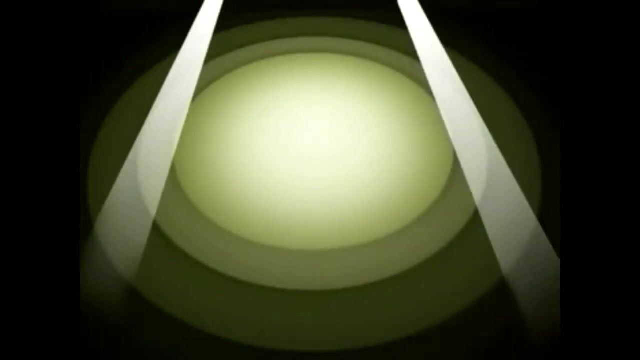 Birds fly. In English, we use letters to make words and words to make sentences. These are what we call the Building Blocks of English. Ladies and gentlemen, let's party tonight. First, let's watch the letter dance. Let's watch the letter dance. 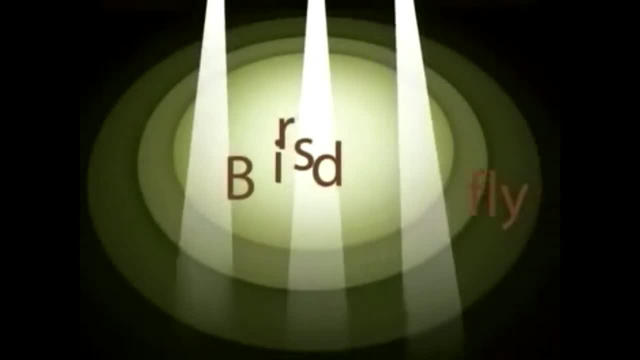 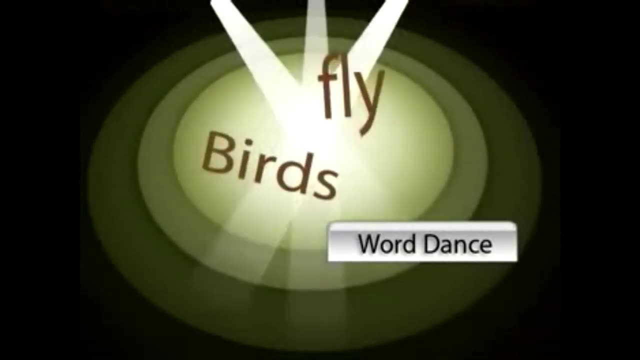 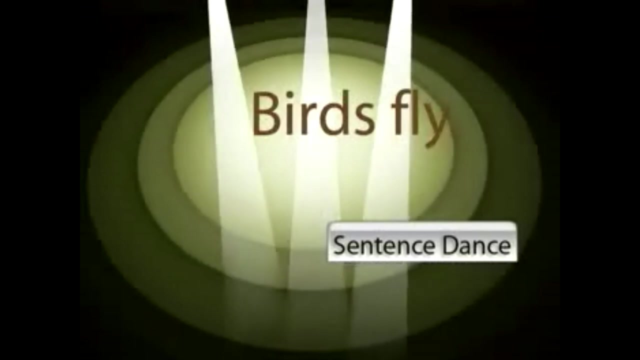 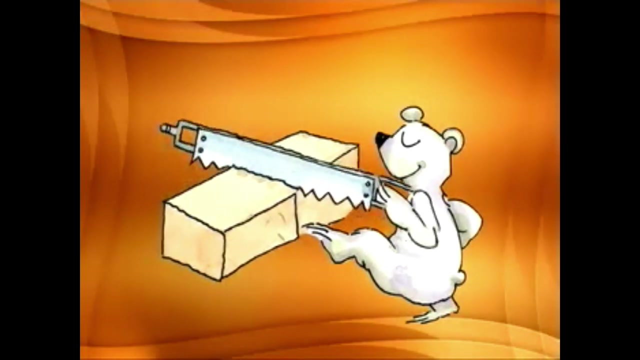 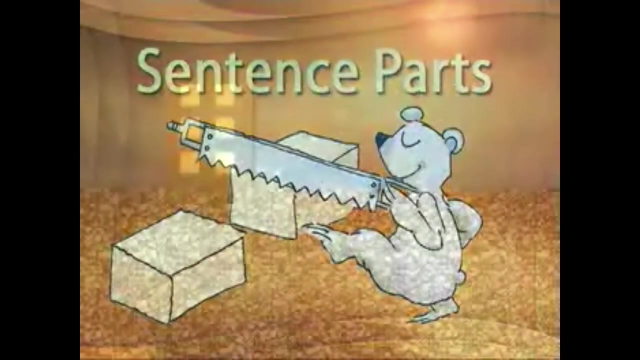 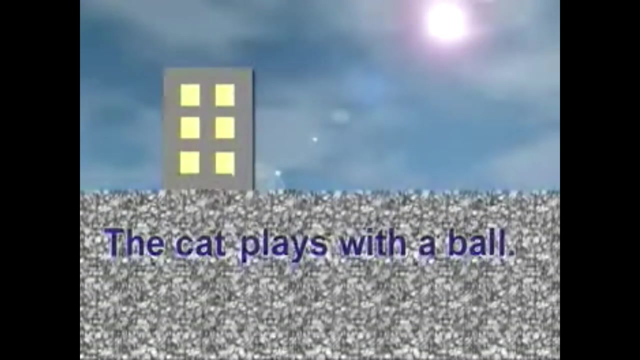 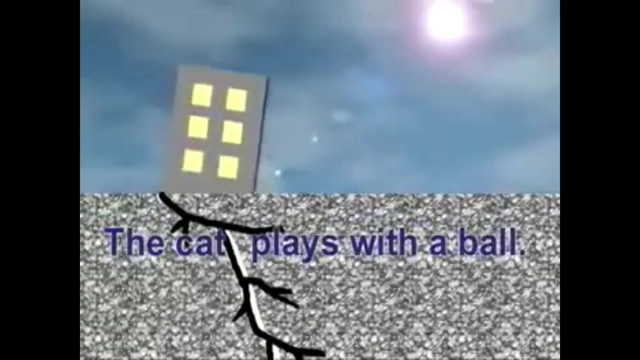 Next the word dance. Last the sentence dance. Yeah, Yeah. Sentence parts. This is a sentence. The cat plays with a ball, Uh-oh. Now the sentence is divided into two parts: The naming part and the action part. 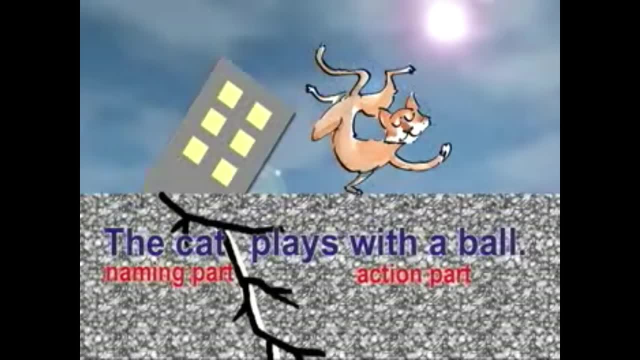 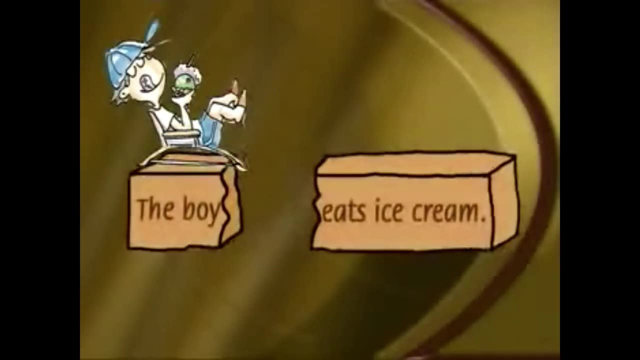 The naming part tells what something is. The action part tells what something does. Let's look at more examples. The action part tells what something does. Let's look at more examples. The boy eats ice cream, And what's he doing? Grandma watches TV. 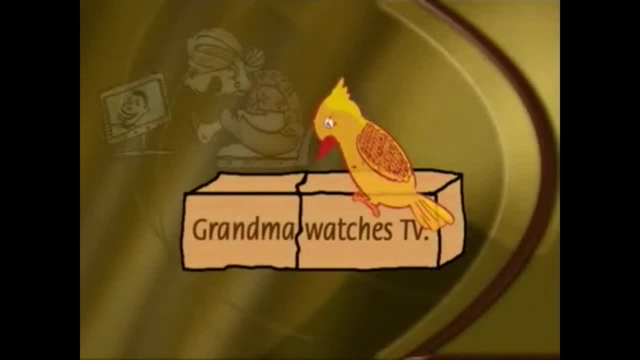 What He plays the ball with a toy in his hand, What He weighs- about 30 to 35 pounds. He startsгу The children are crossing the street. He is greeting each or every other child On the phone, he starts to play video games. 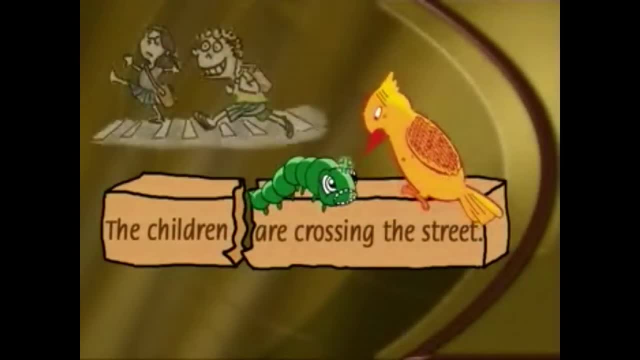 They are playing on the TOMATOMETER screen. Who's at the including screen? The regular, Who at the new screen? You put a name on the board. Who's presenting the chalk? The ich EH. You fill a soap and take a seat back.